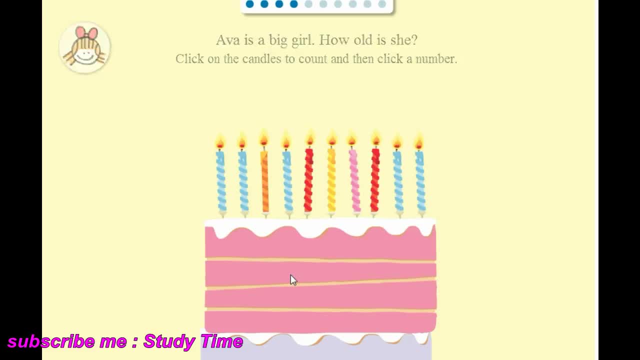 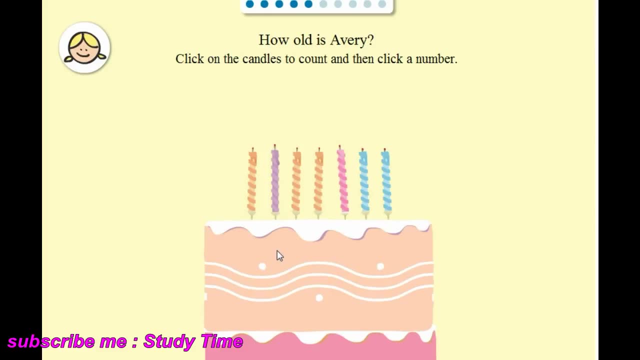 Ten, That's right. How old is Avery? One, Two, Three, Four, Five, Six, Seven, Eight, Nine, Ten, Seven, That's right. How old is Noah? One, Two, Three, Three, That's right. 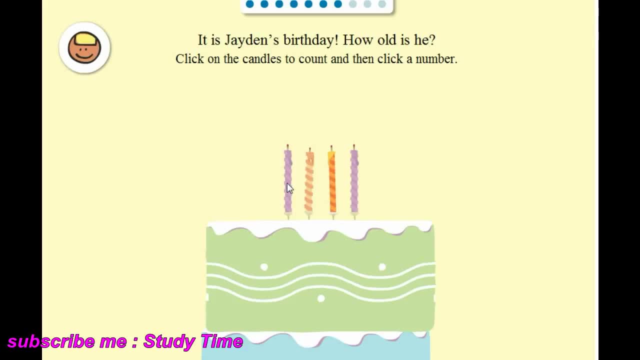 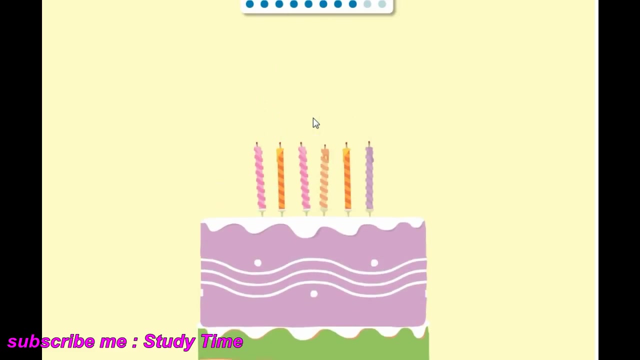 It is Jayden's birthday. How old is he? One, two, three, four, four, That's right. It is Liam's birthday. How old is he? One, one, That's right. Busy is having a birthday party. 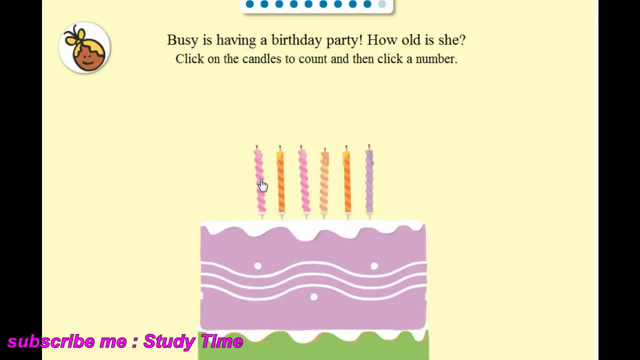 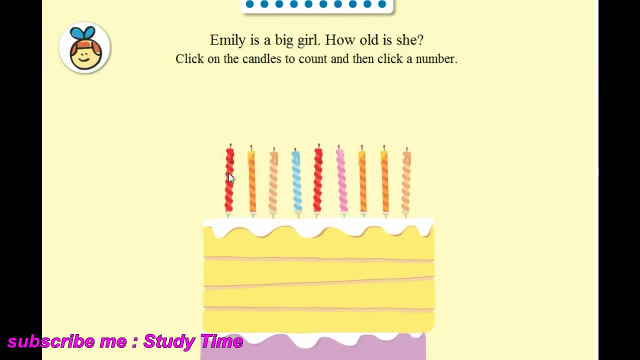 How old is she? One, two, three, four, five, Six, six. That's right, Emily is a big girl. How old is she? One, two, three, four, five, six, Six, Seven, eight, nine, nine. 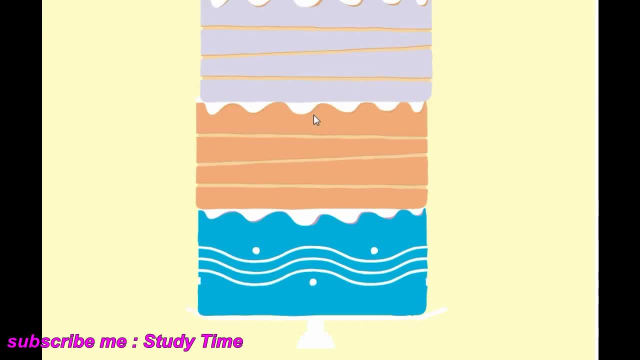 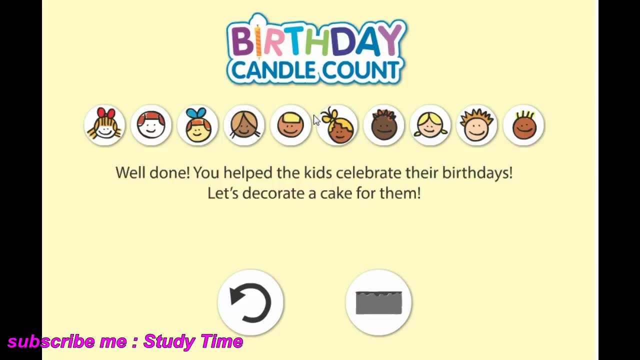 That's right. Well done: You helped the kids celebrate their birthdays. Let's decorate a cake for them.